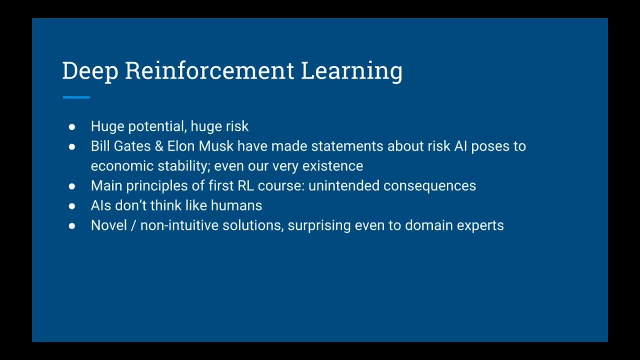 to interact with the real world, and AI has a lot of potential. it also carries with it a huge risk. Bill Gates and Elon Musk have made public statements about some of the risks that AI poses to economic stability and even our existence. As we learned in my first reinforcement learning course, one of the main 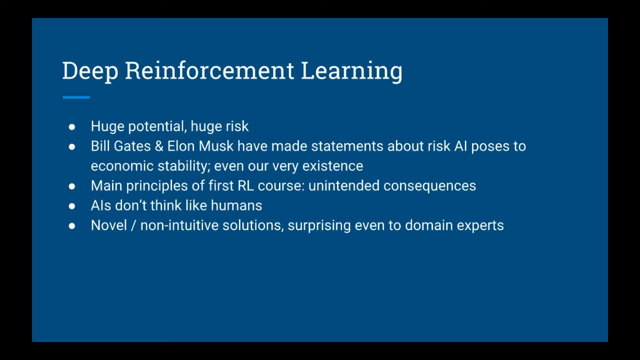 principles of training reinforcement learning agents is that there are unintended consequences when training in AI. AIs don't think like humans, and so they come up with novel and non-intuitive solutions to reach their goals, often in ways that surprise domain experts. humans, who are the 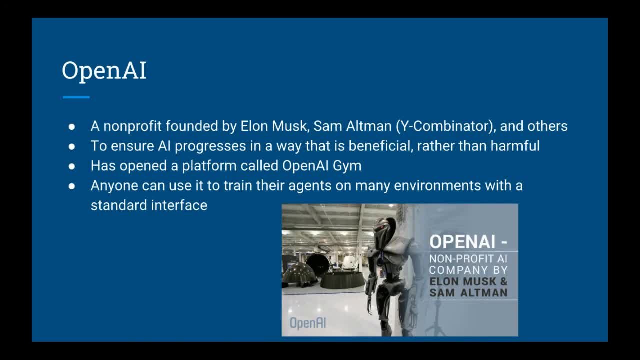 best at what they do. OpenAI is a non-profit founded by Elon Musk, Sam Altman and others in order to ensure that AI progresses in a way that is beneficial rather than harmful. Part of the motivation behind OpenAI is the existential risk that AI poses to humans. They believe that 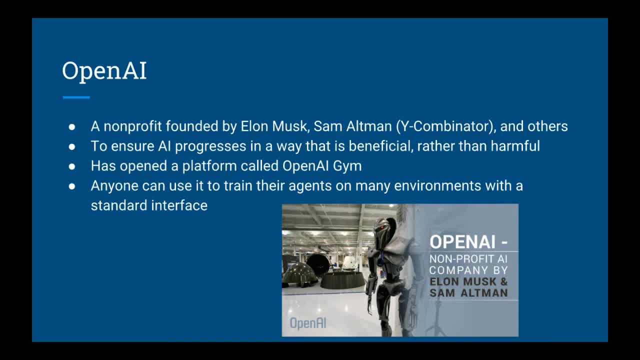 open collaboration is one of the keys to mitigating this risk. One of the great things about OpenAI is that they have a platform called the OpenAI Gym, which we will be making heavy use of in this course. It allows anyone anywhere in the world. 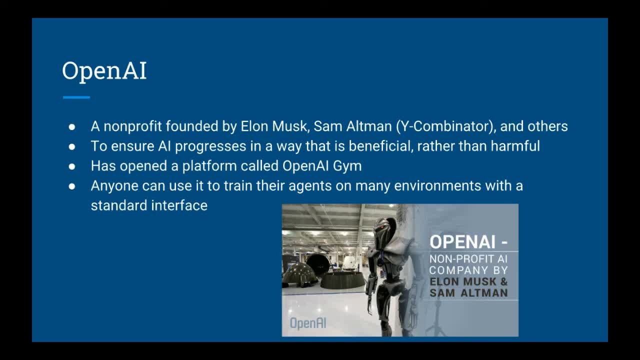 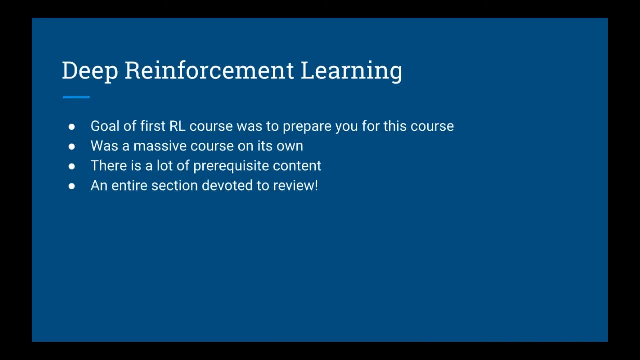 to train their reinforcement learning agents in standard environments. One of the goals of my first reinforcement learning course was to set you up so that you'd be ready for the content in this course At the same time. that course was massive by itself, so you can be sure that if you want to make sure your 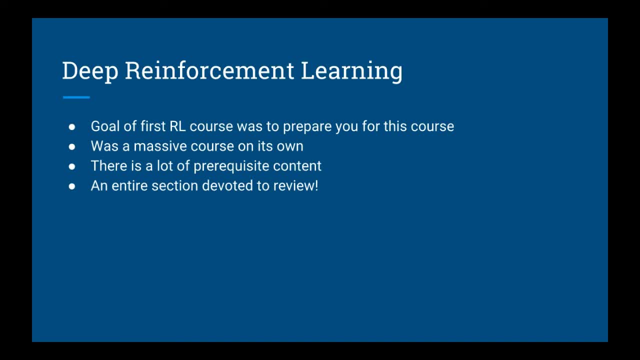 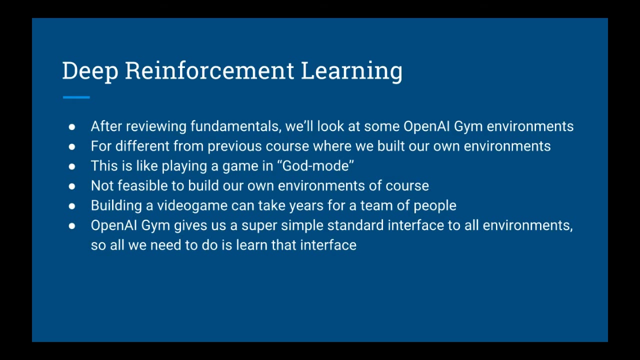 course is ready. for this course, there is a lot of pre-requisite content you'll need to know and have experience with. In fact, I've dedicated an entire section of this course just to go over all the stuff you need to know and to review key principles. What else is in this course After reviewing? 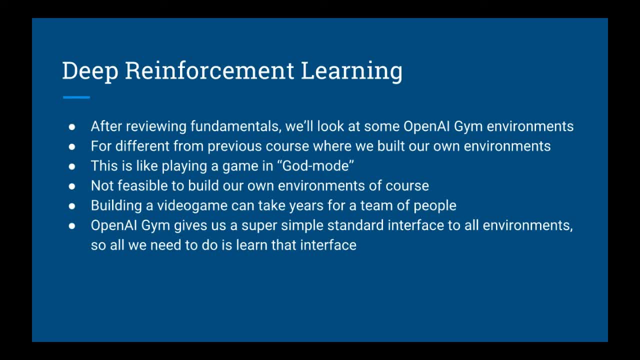 background fundamentals. we'll start building reinforcement learning agents for some select environments in the OpenAI Gym. This is a very different approach from my previous reinforcement learning course. OpenAI Gym gives us a super simple standard interface to all of its environments. so there's. 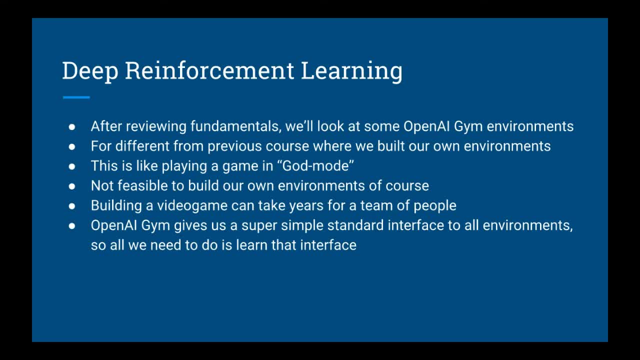 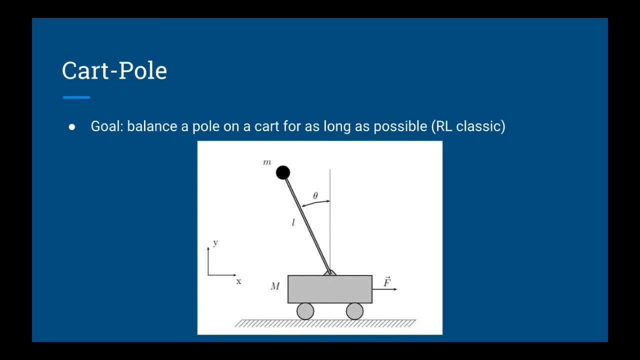 not much thinking we have to do beyond understanding how to interface with it. In this course we'll be training an agent in the cart pole task, also known as the inverted pendulum. This is a reinforcement learning classic. The goal is to balance a pole on top of a. 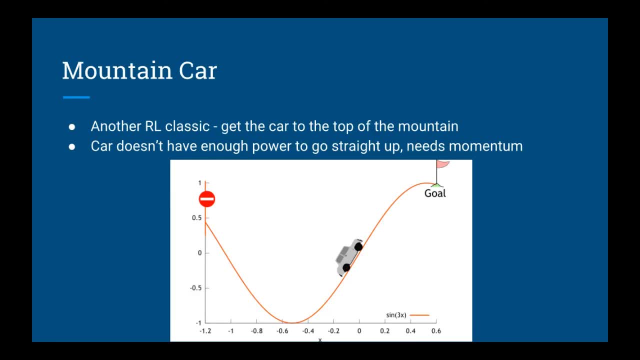 cart for as long as possible. Let's start by finding the correct work points to work at. Let's try this. We'll be training an agent for the mountain cart task. This is another reinforcement learning classic. The goal is to apply the right force at the right time to get the cart to the top of the 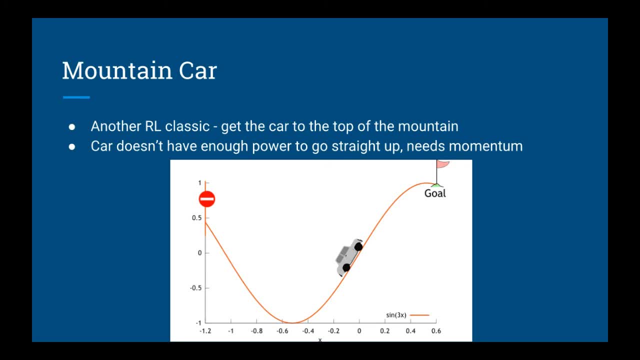 mountain. The car by itself can't generate enough force to push itself up the mountain in one go, so it has to use momentum to swing itself to the top. One key insight about these tasks is that if an agent can learn to solve them, it is. 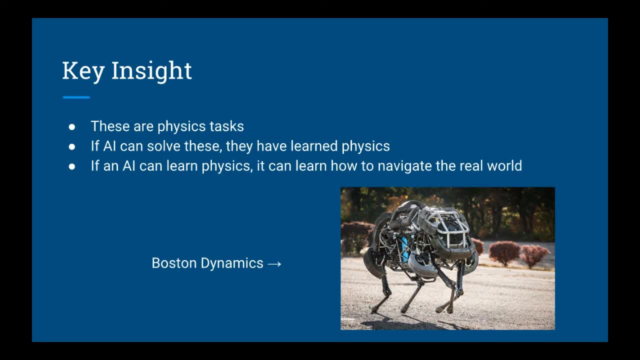 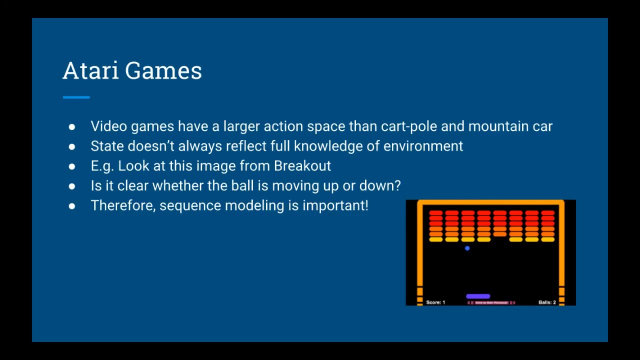 essentially learning physics. If it can learn physics, it can learn how to move about physically in the real world. Here's an example of one of the robots from Boston Dynamics. so you know this stuff really works. There are already companies out there doing it. 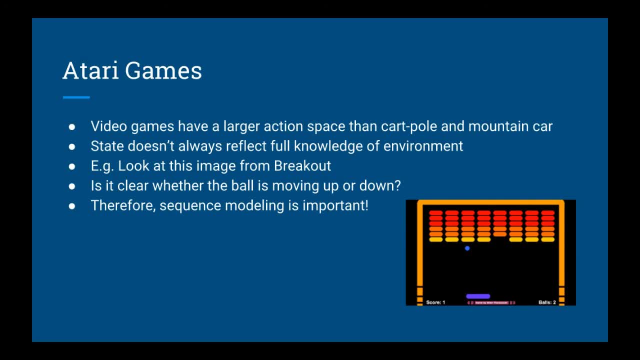 After we look at cart, pole and mountain car, we'll look at one or more Atari games. Playing video games is an essential step we must take in order to build intelligent agents for the real world. Video games contain a larger set of actions than cart, pole and mountain car and the 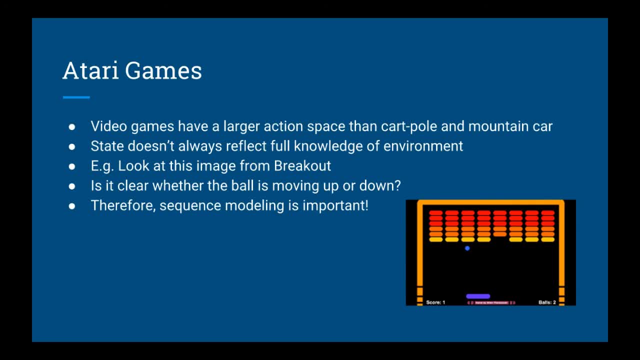 states don't necessarily reflect full knowledge about the environment. For example, look at this picture from the game Breakout. Can you tell whether the car is moving or not? Can you tell whether the ball is moving toward the paddle or away? It's not clear because this is a static image and that's all the information we get from. 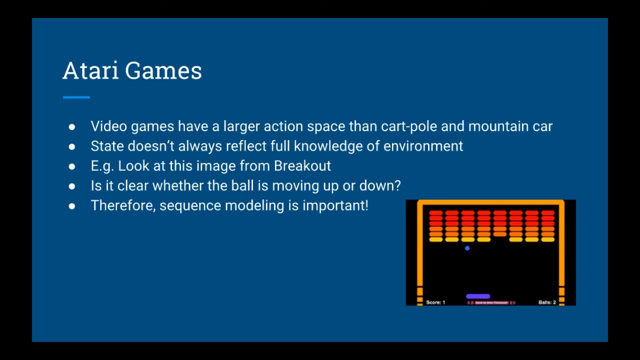 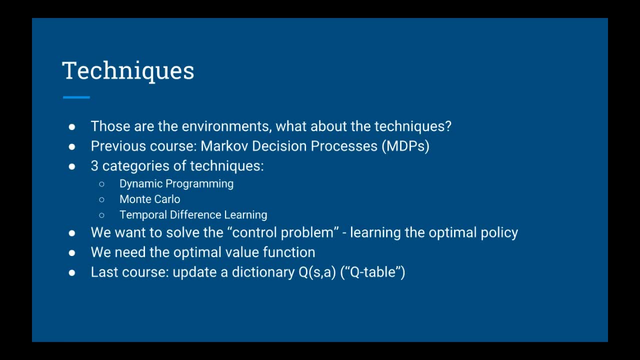 a state. So we'll see that sequence modeling becomes important. But that's enough about what environments we'll be looking at. What about the techniques you'll be learning? In my previous reinforcement learning course, we learned about three main techniques for solving Markov: Decision Processes, or MDPs. 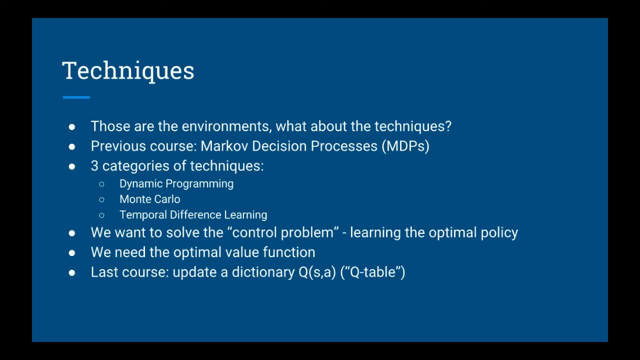 These were Dynamic Programming, Monte Carlo and Temporal Difference Learning. We learned that what we want to do eventually is solve what's called the control problem. That means learning the optimal policy so that whenever we're in a state, we take the 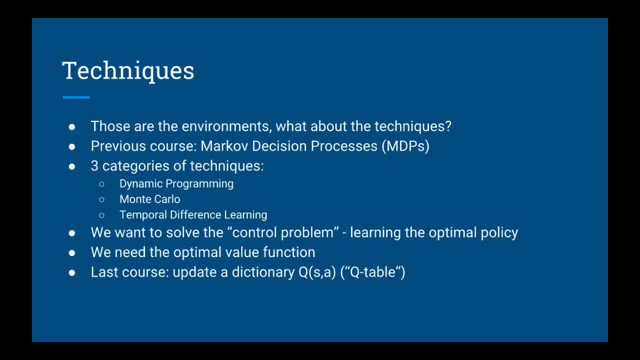 best action based on that state. We learned that in order to find the optimal policy, one of the main ingredients is the optimal value function. We saw that by keeping a dictionary that maps states and actions to values, called a Q-table. we can eventually find the optimal policy by iteratively updating it. 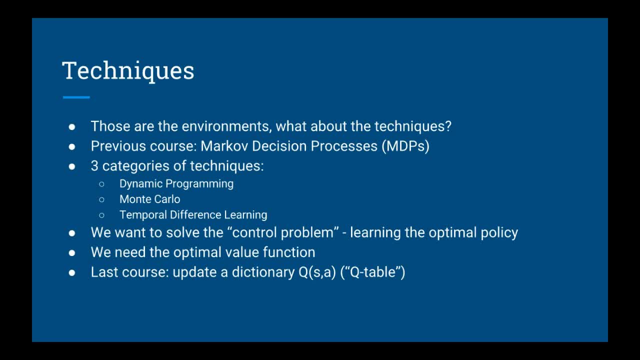 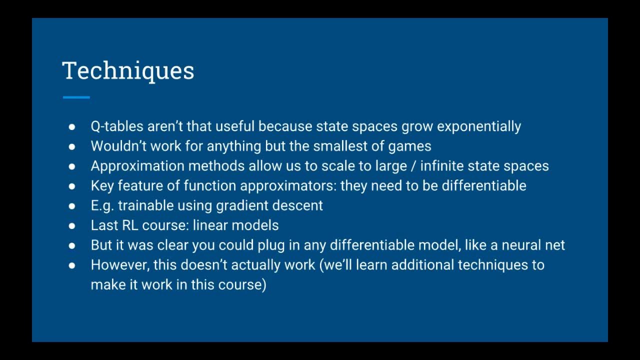 Then we saw that Q-tables aren't that useful, because state spaces generally grow exponentially, and so we wouldn't be able to use them for anything but the smallest of games. We then looked at approximation methods, which allow us to scale to large and possibly infinite. 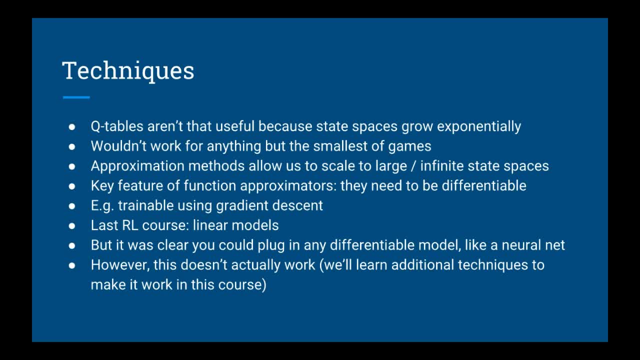 state spaces. One key feature of the function approximators we use for reinforcement learning is that they are differentiable. In other words, we can train them to be different. In other words, we can train them to be different. We can train them using gradient descent, which you learned about in earlier deep learning. 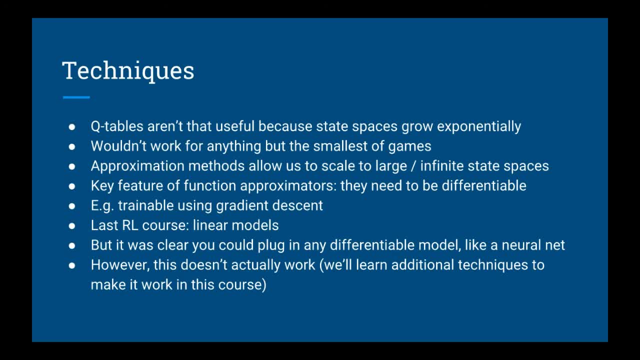 courses. In my first reinforcement learning course we stuck to linear models, but I stated that you could plug and play any kind of differentiable model like a neural network. In this course, you'll learn that this is not necessarily the case. 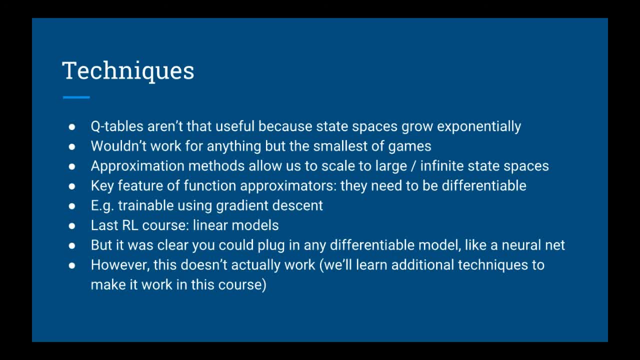 In fact, plugging in a deep neural network into the agents, as we've been building them, just won't work. You can get the syntax just right and the neural network might appear to be approximating some function, but it just won't work as intended. 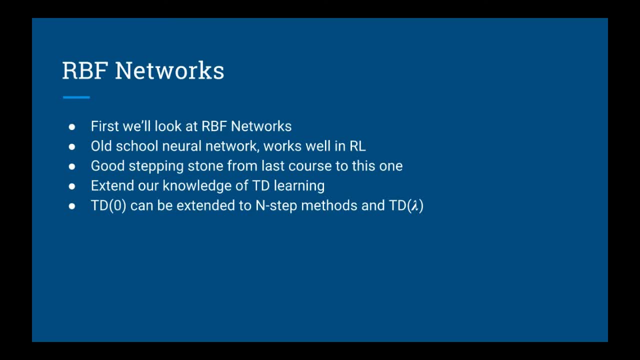 In this course, we'll start by looking at RBF networks. These are old school, but they work well in reinforcement learning. They also fit into the context of what we did in the last course, and so they provide a good stepping stone to the more advanced topics in this course. 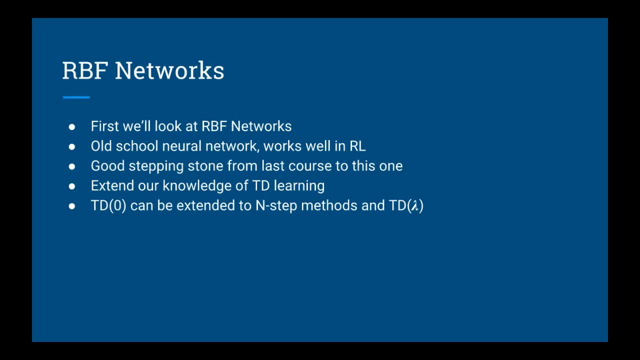 After we learn how to build an RBF network, we'll extend our knowledge of temporal difference learning. So far we know about TD0, but we'll see how the idea behind TD0 can be extended to n-step methods and the more general TD lambda. 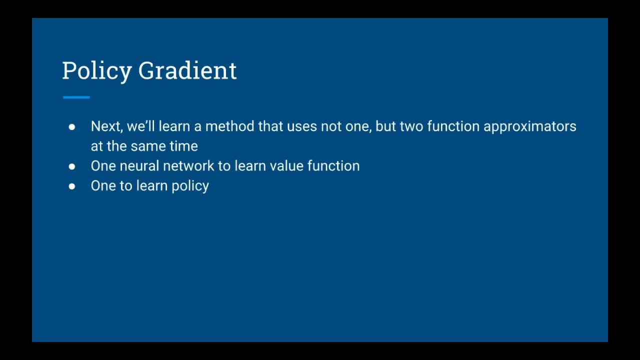 After that, we'll look at a method that uses not one but two function approximators at the same time. In particular, we'll be using one neural network to learn the value function and one neural network to learn the policy. This is called the policy gradient method.